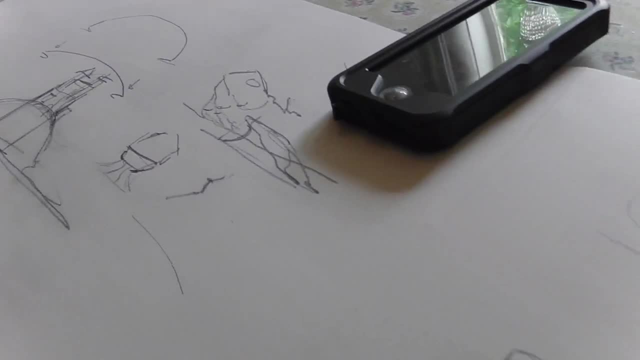 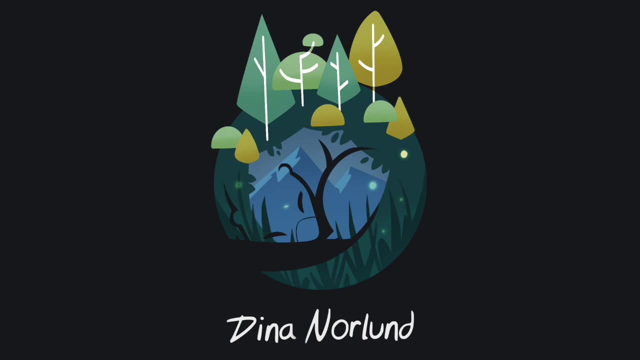 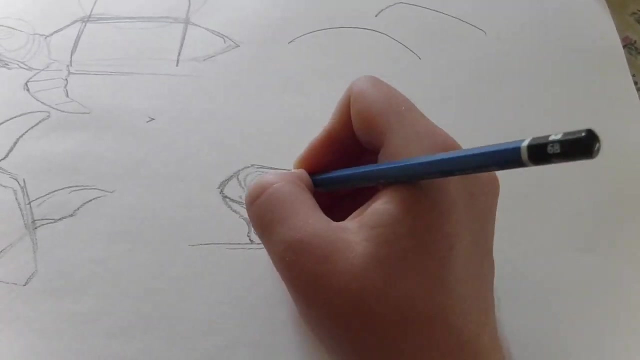 Hello everyone and welcome back to my art channel. Today we are doing something a little bit different and that is a sand sculpture. I haven't been doing this on my art channel yet, but I do really love working with sculpture and doing sculpture stuff and every year, me and my family, we go on the beach and we do. 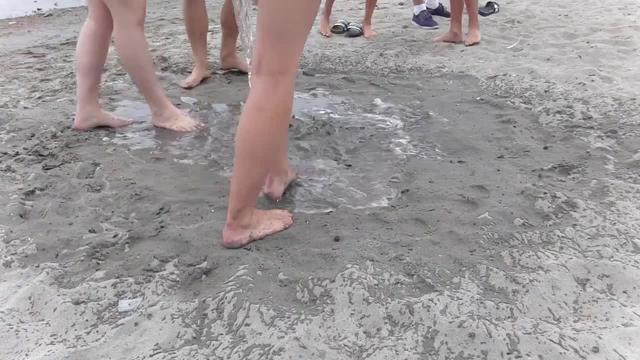 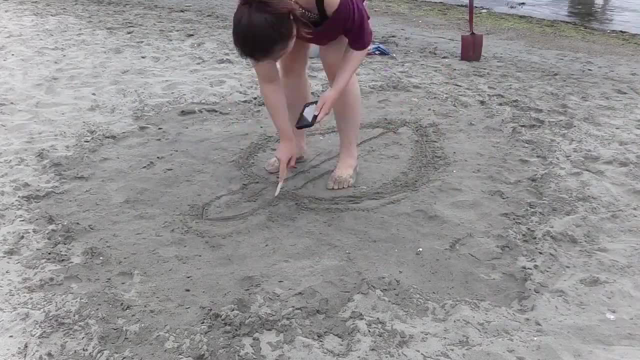 sand sculpture and usually it is with a competition. that happens in the festival week here at my cabin in Norway and we tend to do it with that, but this year it was rainy and they moved it, so we ended up doing our own little sculpture alone on the beach another day and 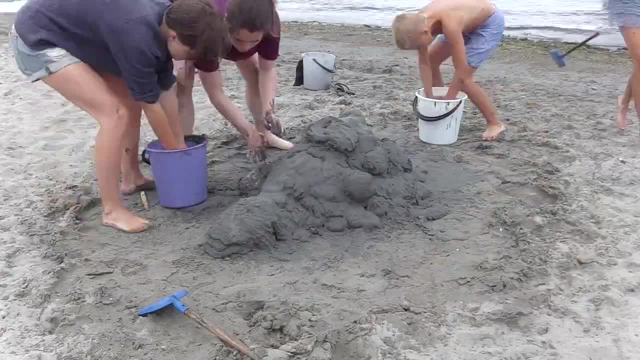 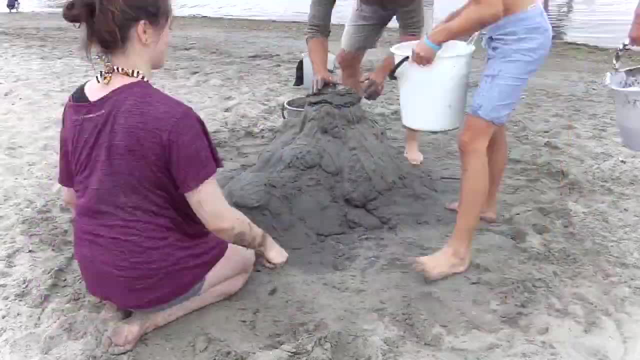 we spent a lot more time than we usually are allowed when we are in the competition. So since we had a lot more time, I thought I would record it and post it up on YouTube, just to show you guys how we actually do sand sculptures, because you would think that we just 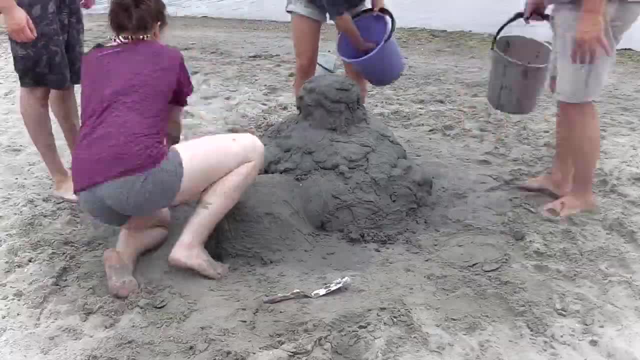 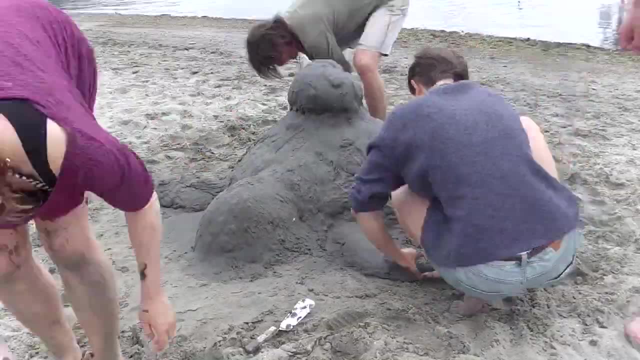 use buckets and we put sand in it and it kind of shapes like a castle. But actually we go out in the ocean and we get some sand that's been in the water for a while and somehow that picks up clay as well, so when we put it on the beach, you can see it's a lot darker. 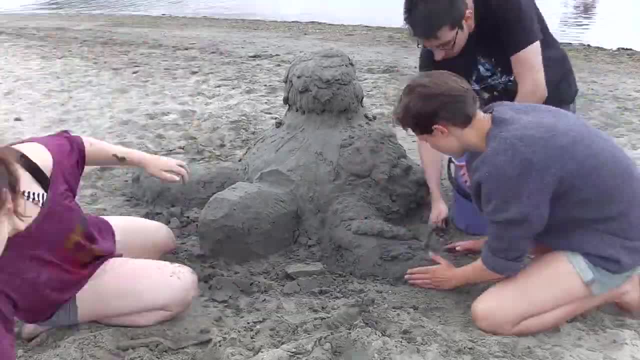 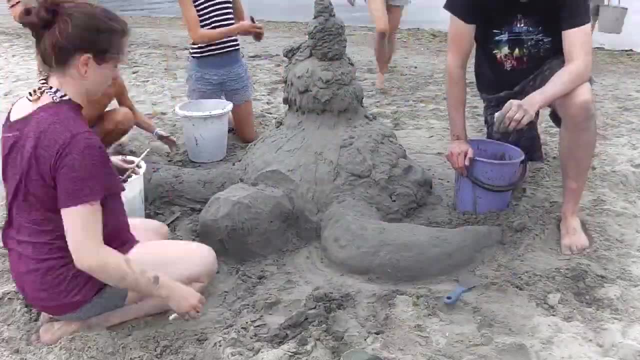 and it's a lot easier to shape. so it's almost like clay, but still sand, so it still dries out very quickly. so we try to keep it wet. but it was harder at the end to keep the details because of the the sand. but if you ever do a sand sculpture on the beach, I would recommend getting the sand. 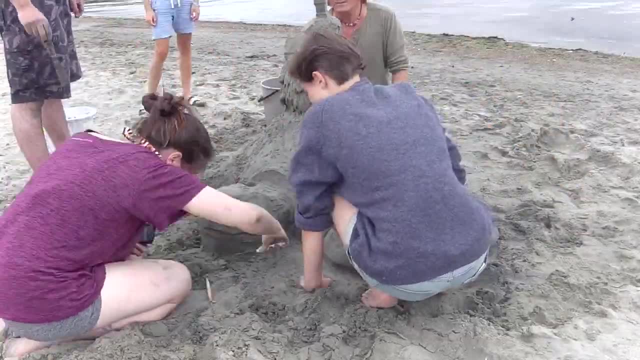 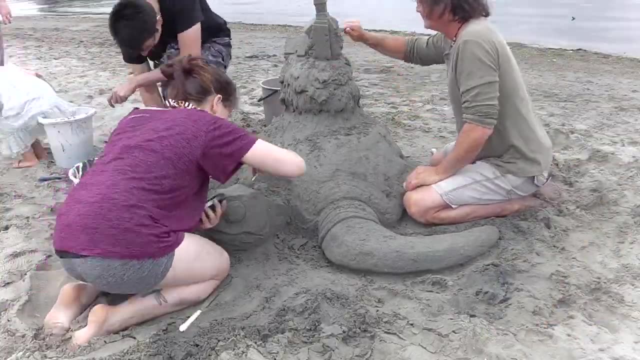 out in the ocean and just use that, because it's a lot easier and it's a lot more fun. So, as you can see, I am the one in the pink or purple t-shirt. If you haven't seen me before, this is this is me and my family and my boyfriend and some random. 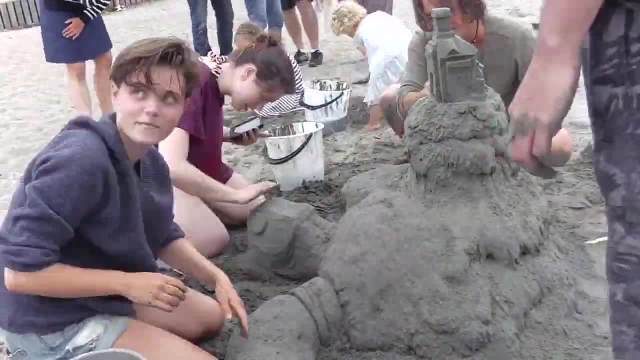 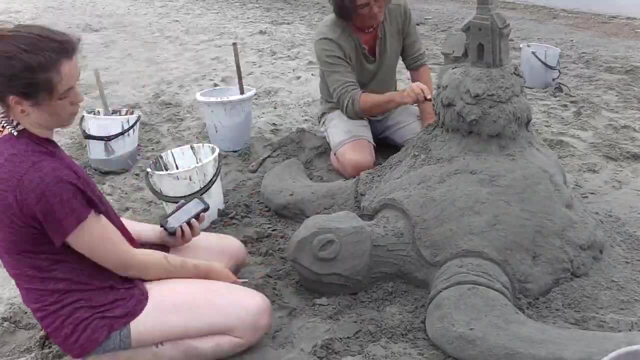 audience walking around in the background. My dad is responsible for the castle at the top and I'm doing the turtle and we ended up only being us two at the end because the people got bored, because we was three hours on this and it was a lot of fun. but I understand when people don't.